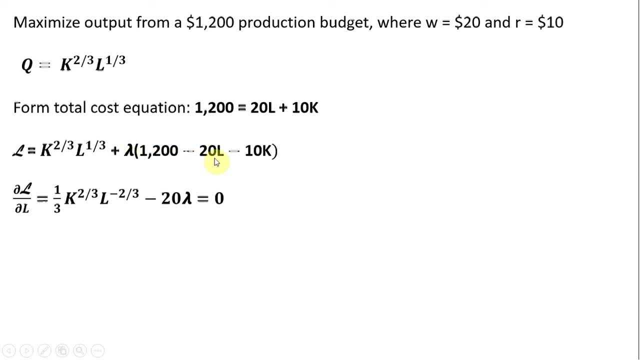 Lambda multiplied by minus 20L, the partial derivative of that will just be minus 20 lambda. I don't have to worry about lambda times $1,200 or lambda multiplied by minus 10K. neither of those terms have an L in it, so they're just going to be treated as a zero or a constant when we take a partial derivative. 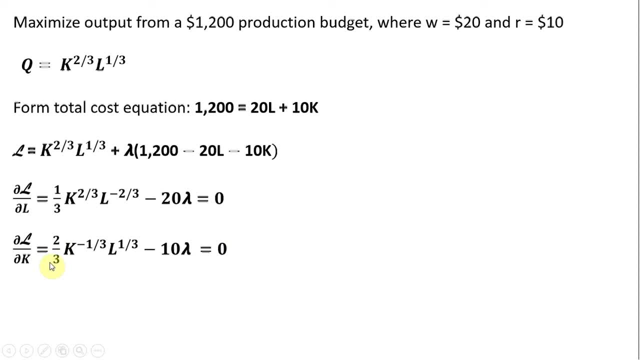 The next partial derivative is the partial derivative of the Lagrangian with respect to capital. The 2 thirds here on the K term gets brought down in front. 2 thirds minus 1 leaves us K raised to the minus 1 third power. 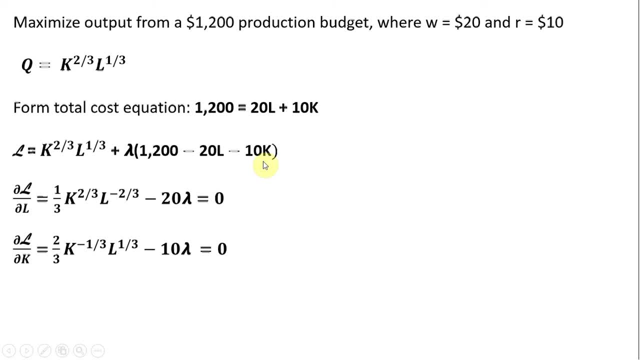 And then lambda. multiplied by minus 20L, The partial derivative of that is just minus 10 lambda And one more partial derivative. We will take the partial derivative of the Lagrangian with respect to lambda. We'll get back what is in the parentheses here: the cost constraint. 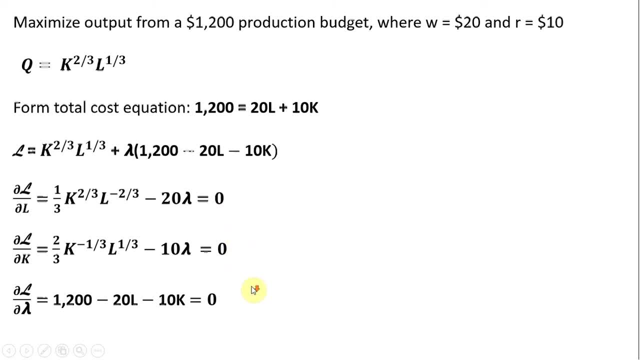 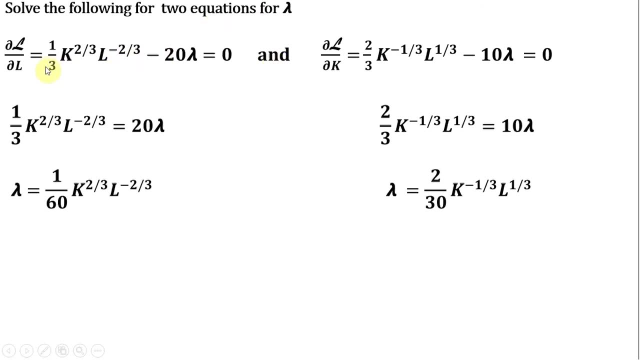 All these partial derivatives are set equal to zero. The next step is we are going to solve our first two partial derivatives for lambda. So we're going to take this partial derivative result and solve it for lambda, Moving 20 lambda over to the right-hand side and then dividing through by 20, we will get this result. 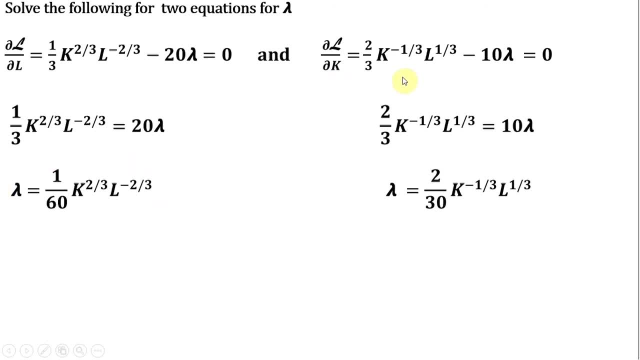 And then this next partial derivative. we'll do the same thing, Moving 10 lambda over to the right-hand side and dividing through by 10, we'll get this result. I'm going to set both of these lambda equations equal to each other. 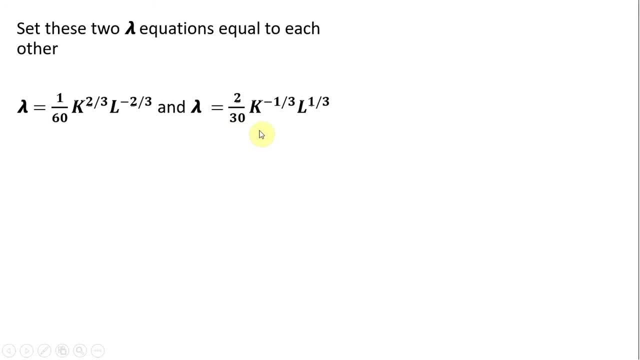 This is what we found on the last slide, Setting lambda equal to lambda. And now simplifying. The first thing I did was I multiplied both sides through by 60.. So 60 times 2 is 120.. Divided by 30 gives us 4.. 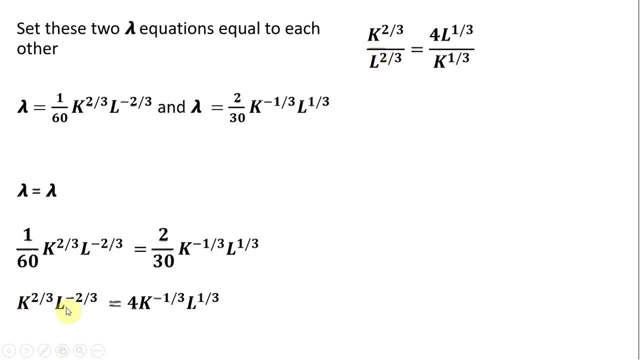 Following the rules of exponents, on the left-hand side, we're going to move this L to the minus 2 thirds into the denominator, And that will then become L raised to the 2 thirds power, And we'll do a similar thing on the right-hand side.